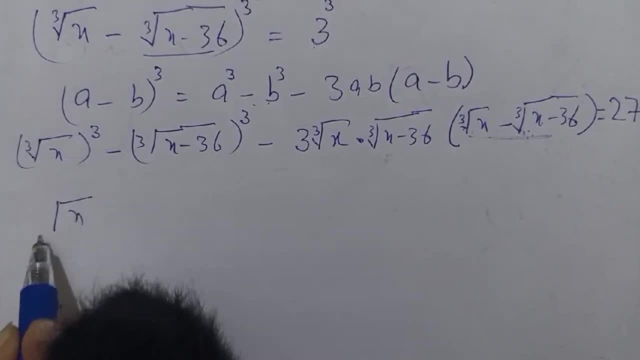 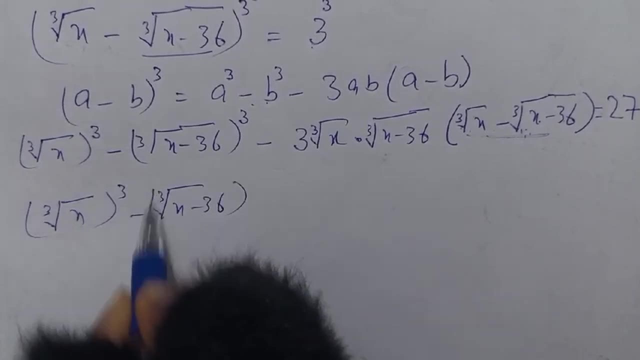 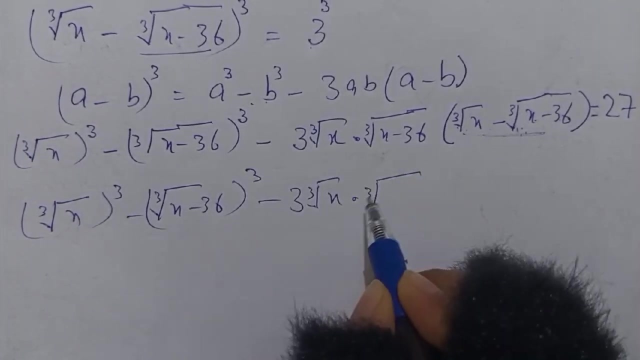 So this will become a cube root of x raised to power 3 minus cube root of x minus 36, raised to power 3 minus 3, cube root of x into cube root of x minus 36 and is equal to 3, is equal to 27.. 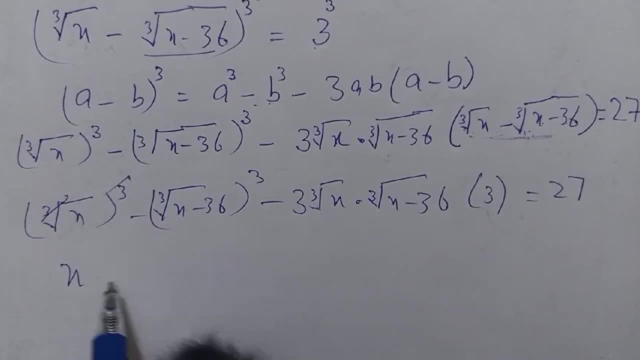 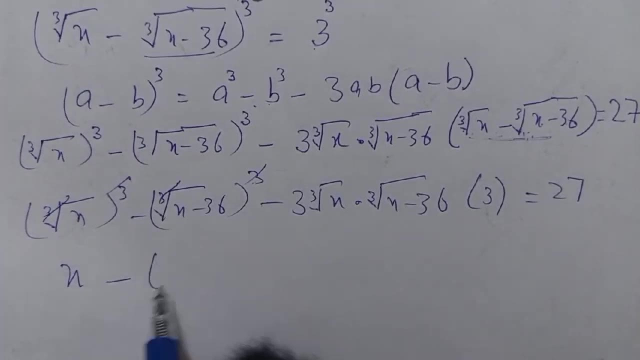 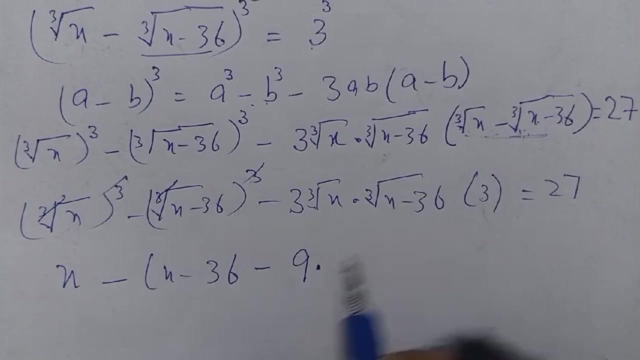 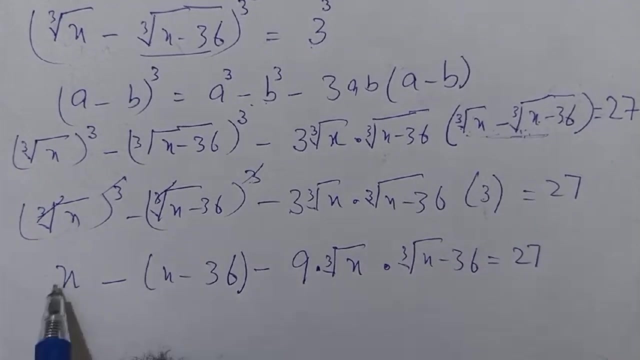 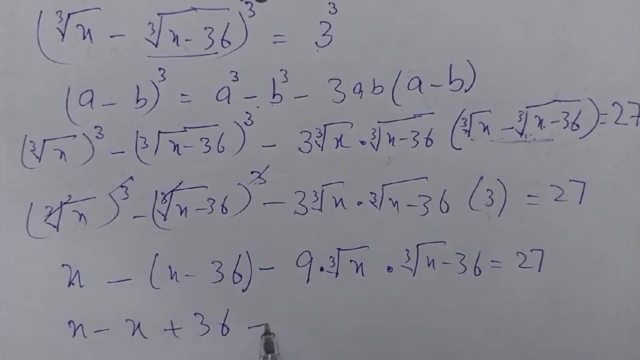 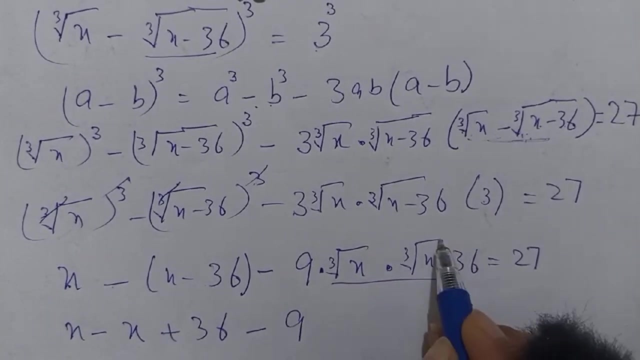 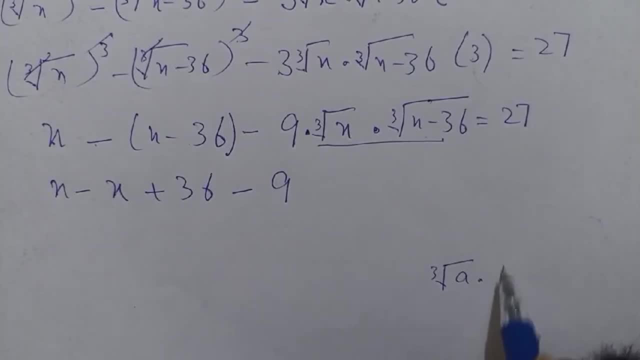 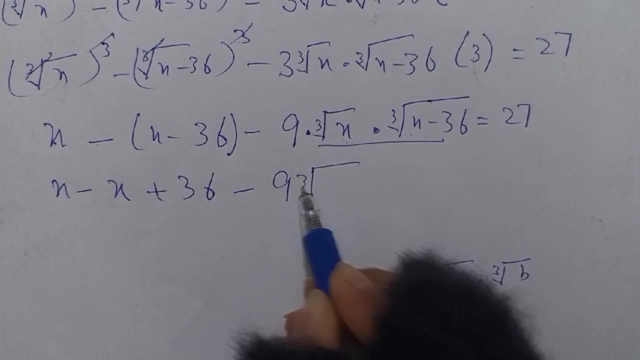 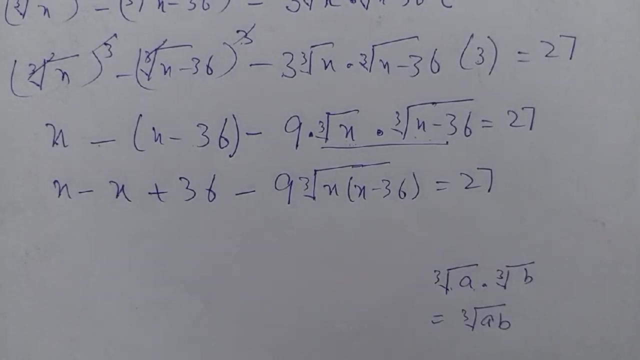 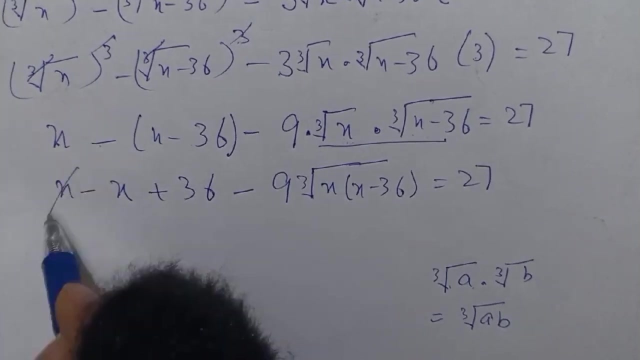 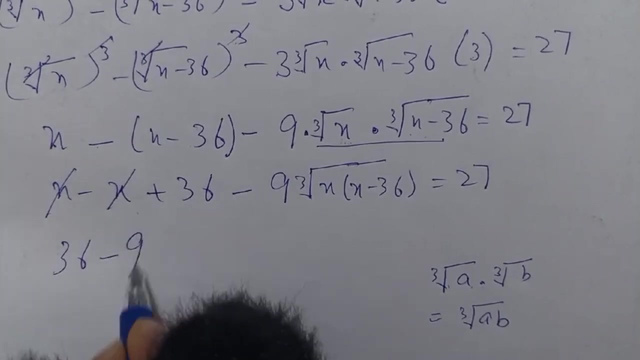 cube root of a. multiply cube root of b. it's equal to cube root of a- b, so we apply this property on this value. then this will become a cube root of x. multiply x minus 36 is equal to 27, and so this will be cancelled. we just get 36 minus 9. cube root of x. multiply x- 6- x. 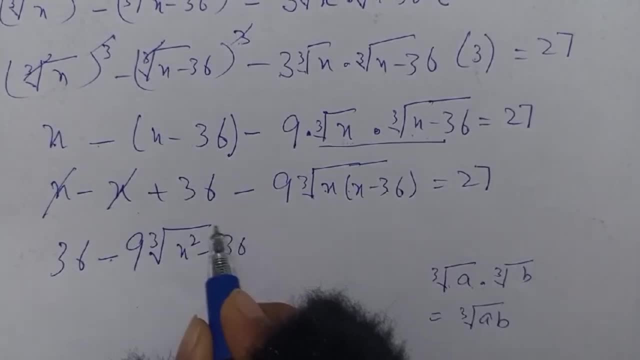 so this will be cancelled. we just get 36 minus 9 cube. root of x multiply x- 6 x. so this will be cancelled. we just get 36 minus 9 cube. root of x multiply x- 6 x. cube minus 36 x is equal to 27, so we cube root of x multiply x- 6 x square minus 36 x is equal to 27, so we cube root of x multiply x, 6 x square minus 36 x is equal to 27, so we subtract 36 on both sides of this equation. 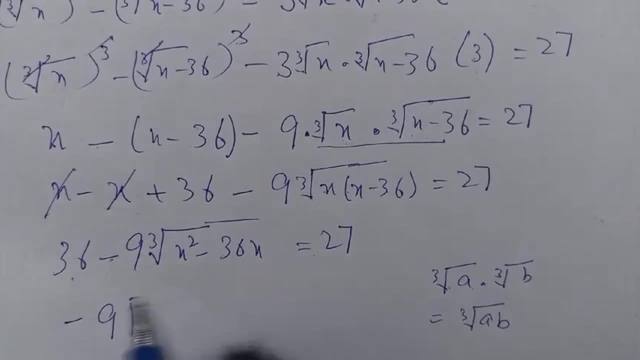 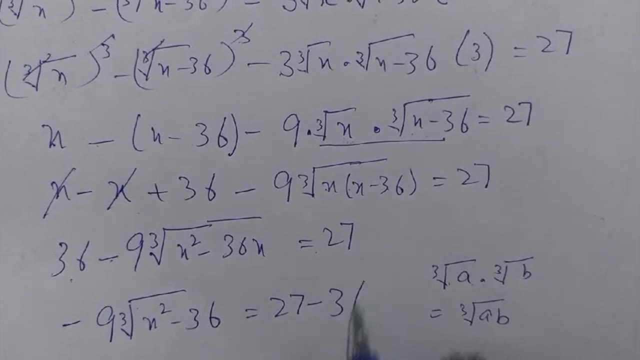 subtract 36 on both sides of this equation. subtract 36 on both sides of this equation, then we get minus cube root of x squared. then we get minus cube root of x squared, then we get minus cube root of x squared. minus 36 is equal to 27, minus 36 and 27. 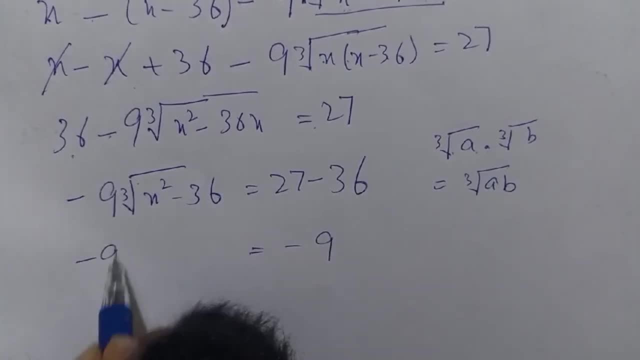 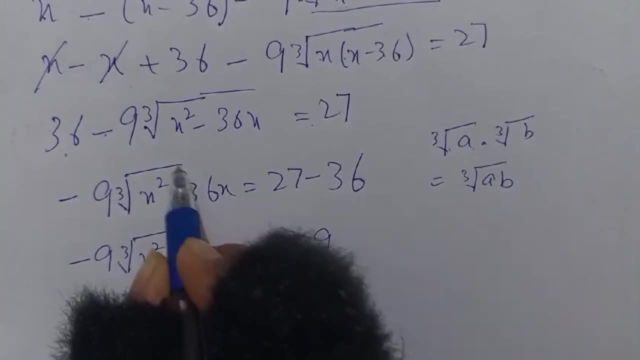 minus 36 is equal to minus 9, and this is a minus 9. cube root of x squared minus minus 9. cube root of x squared minus minus 9. cube root of x squared minus 36: x. here is x. okay, now we divide minus 9. 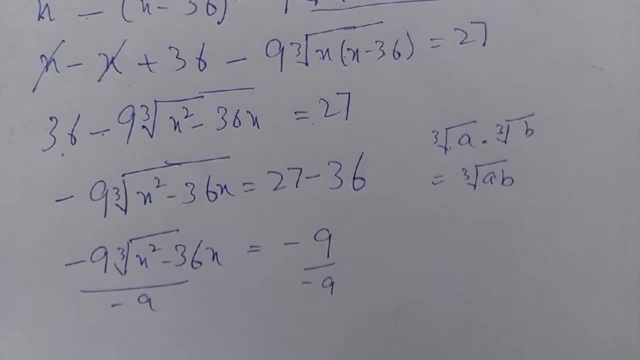 36 x. here is x. okay. now we divide minus 9: 36 x. here is x. okay, now we divide minus 9 on both sides of this equation, then we on both sides of this equation, then we on both sides of this equation, then we will get. 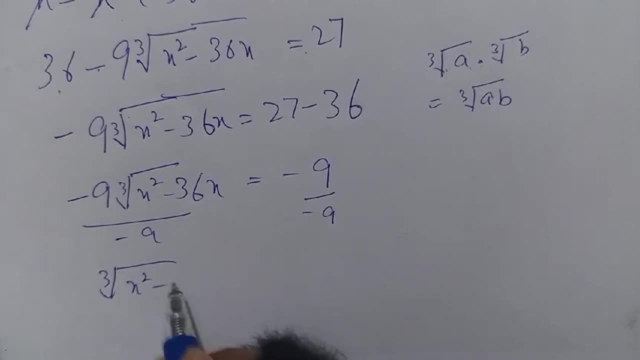 will get. will get. cube root of x, squared minus 36, is equal to 1. cube root of x, squared minus 36, is equal to 1. cube root of x, squared minus 36, is equal to 1. taking a cube on both sides of this. 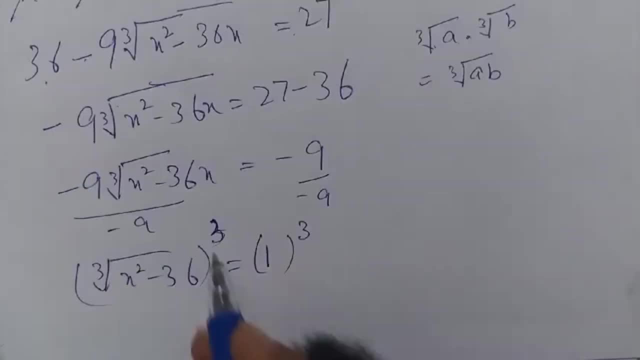 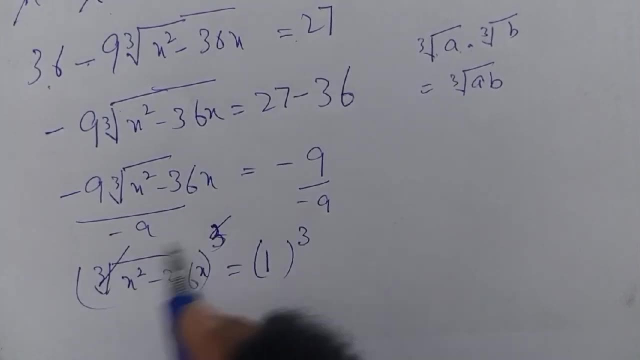 taking a cube on both sides of this. taking a cube on both sides of this equation, and after that, we cancel this, we equation. and after that we cancel this, we equation. and after that we cancel this. we just get. we cancel this and we get x. just get, we cancel this and we get x. 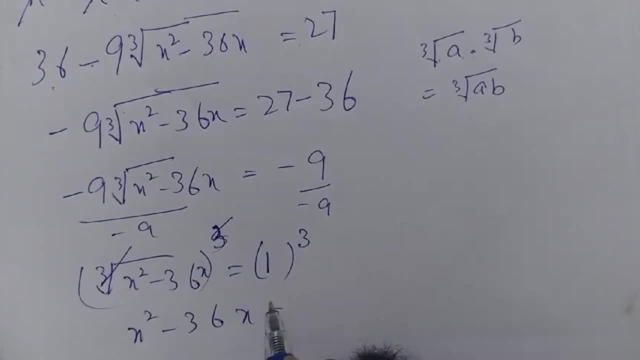 just get. we cancel this and we get x. square minus 36: x is equal to 1 is equal. square minus 36: x is equal to 1 is equal. square minus 36: x is equal to 1 is equal to 1. so divide this equation by x and. 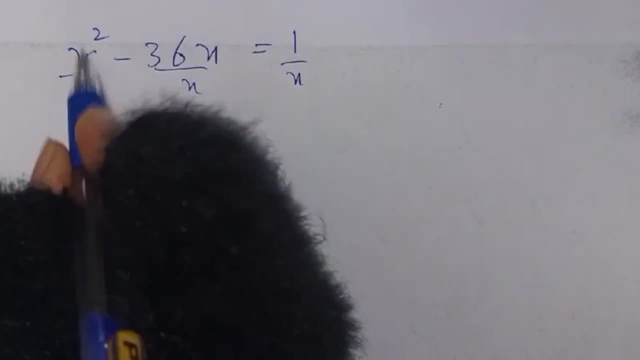 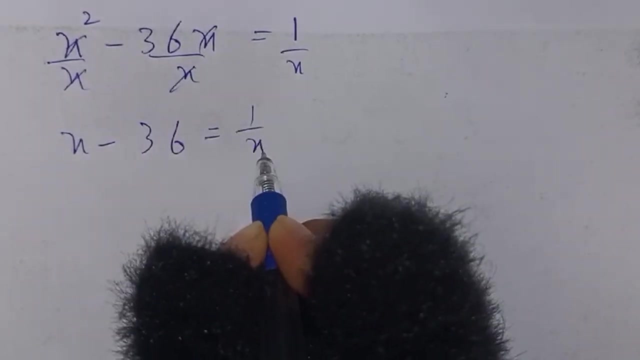 to 1, so divide this equation by x. and to 1, so divide this equation by x. and after cancellation: we just get X minus after cancellation, we just get X minus. after cancellation, we just get X minus. 36 is equal to 1 by X if we shift this 1. 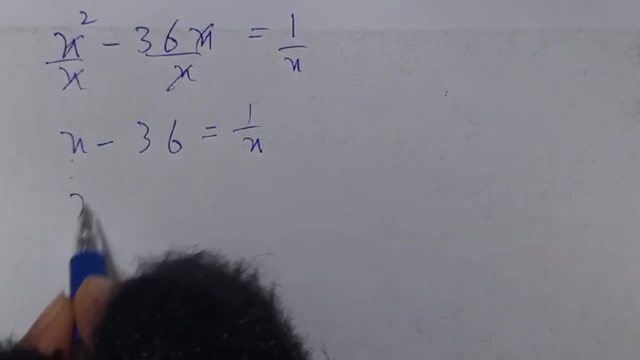 36 is equal to 1 by X. if we shift this 1, 36 is equal to 1 by X. if we shift this 1 by X to left-hand side, then this will by X to left-hand side, then this will by X to left-hand side, then this will become a X minus 1 by X. and if we add 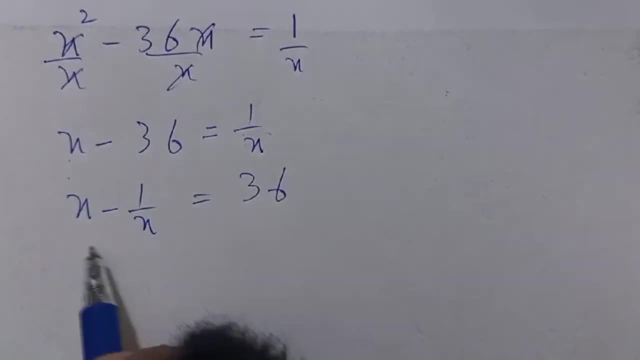 become a X minus 1 by X. and if we add, become a X minus 1 by X. and if we add 36 on both sides, then we get 36, so it's a 36 on both sides, then we get 36, so it's a. 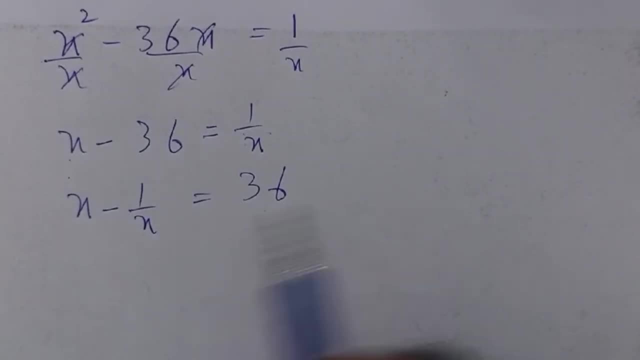 36 on both sides. then we get 36. so it's a value of X minus 1 by X, which is 36, but value of X minus 1 by X, which is 36, but value of X minus 1 by X, which is 36. but in our question we just find the value. 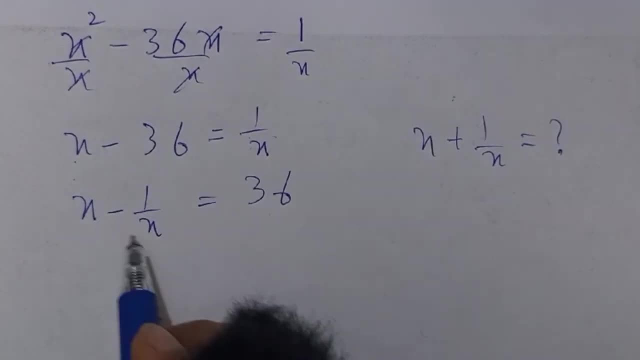 in our question we just find the value. in our question we just find the value of X plus 1 by X. so if we take a square of X plus 1 by X, so if we take a square of X plus 1 by X, so if we take a square on both sides of this equation and here 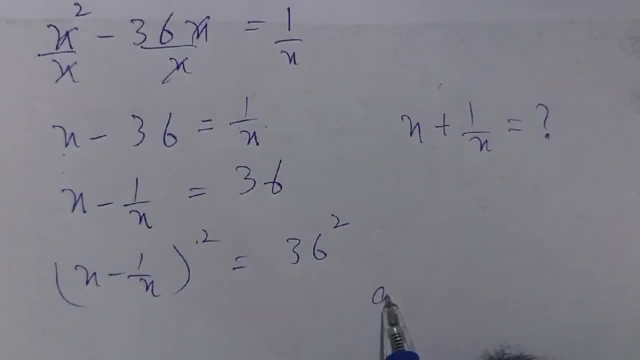 on both sides of this equation and here, on both sides of this equation, and here, we use a formula a square which is a. we use a formula a square which is a. we use a formula a square which is a minus B: whole square is equal to a. 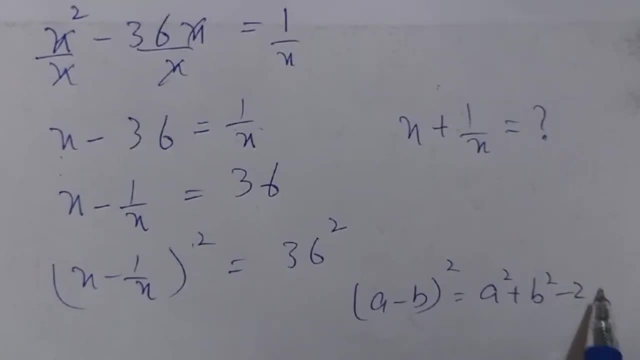 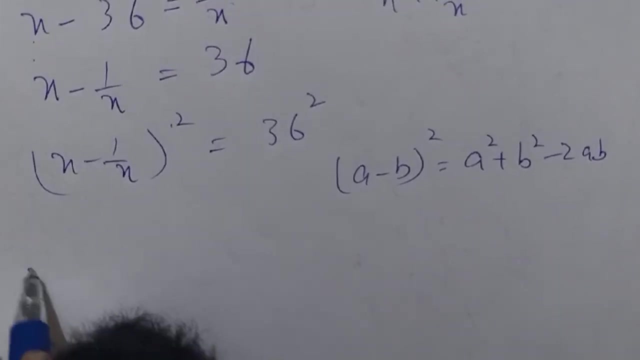 minus B, whole square is equal to a minus B whole square is equal to a square plus B square minus 2 a P. so this square plus B square minus 2 a P, so this square plus B square minus 2 a P. so this will become: 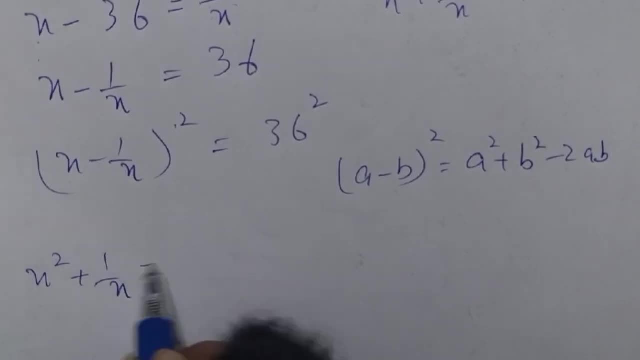 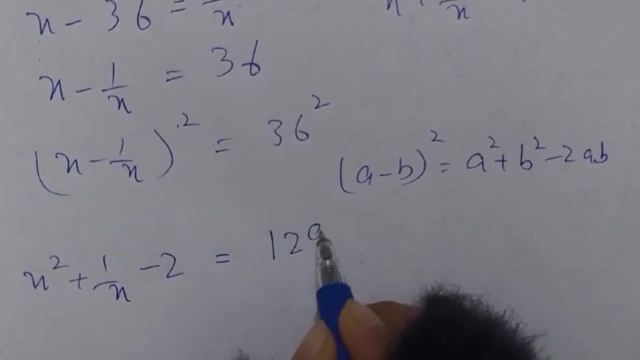 will become will become: our X square plus 1 by X minus 2 is our X square plus 1 by X minus 2 is: our X square plus 1 by X minus 2 is equal to n. 36. here is 1296 if we add 2. 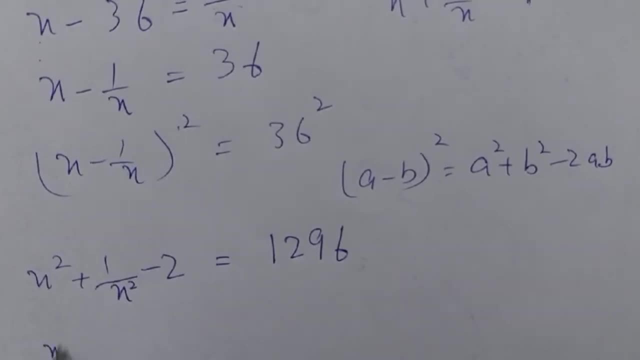 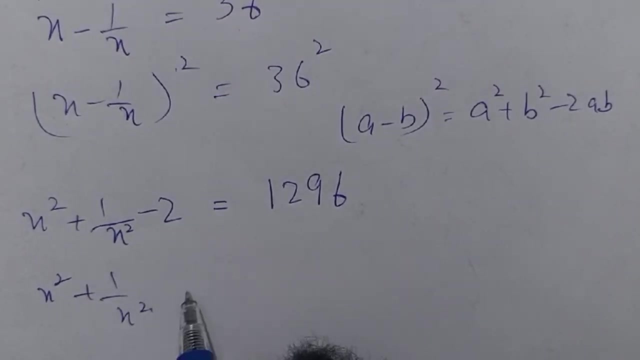 equal to n 36, here is 1296. if we add 2: equal to n 36, here is 1296. if we add 2 on both sides of this equation, then we on both sides of this equation, then we on both sides of this equation, then we get X square plus 1 by X square is: 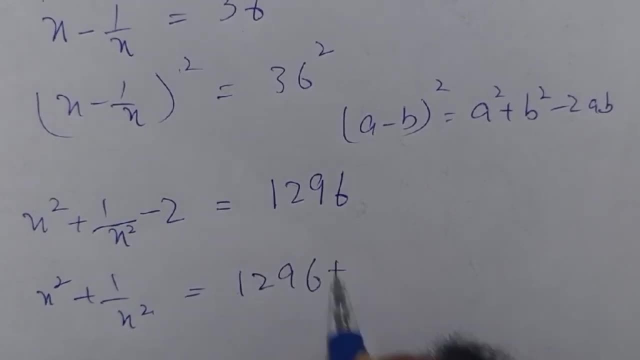 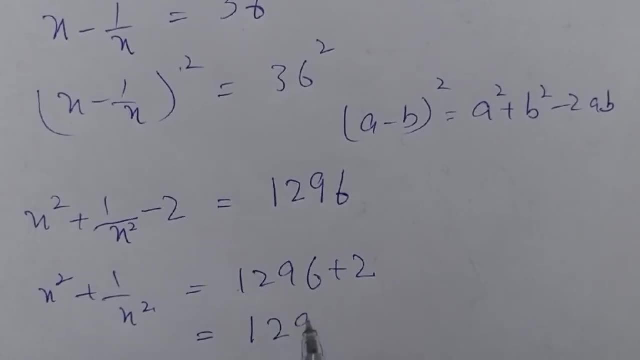 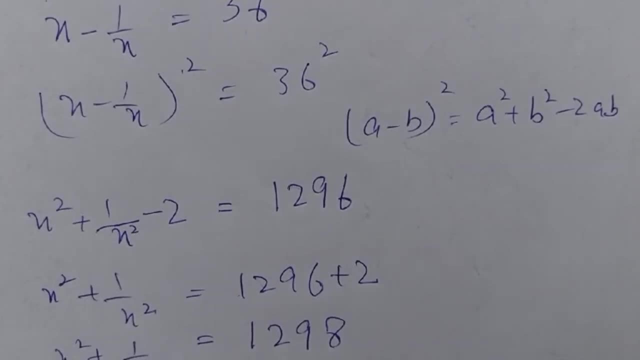 equal to 1296 x here plus 1 by x. equal to 1296 x here plus 1 by x. here is the value of X square plus 1 by X. and here is the value of X square plus 1 by X. and here is the value of X square plus 1 by X. and we find the value of X plus 1 by X. so 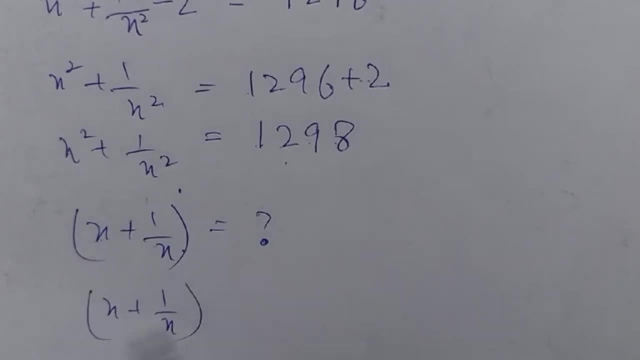 we find the value of X plus 1 by X. so we find the value of X plus 1 by X. so X plus 1 by X, whole square, as you know, X plus 1 by X, whole square, as you know. X plus 1 by X, whole square, as you know, it's equal to X square plus 1 by X. 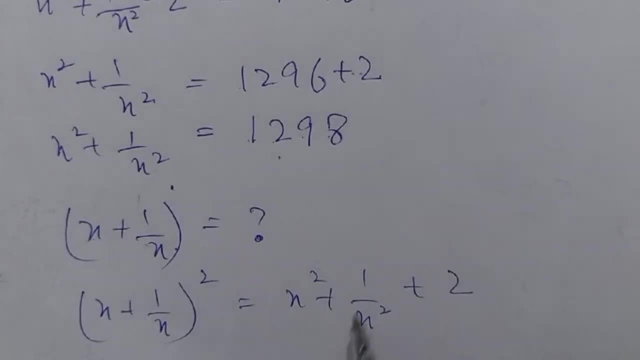 it's equal to X square plus 1 by X. it's equal to X square plus 1 by X, square plus 2, and X square plus 1 by X is square 2, and X square plus 1 by X is square 2, and X square plus 1 by X is equal to 1298. so we put this value 1298.